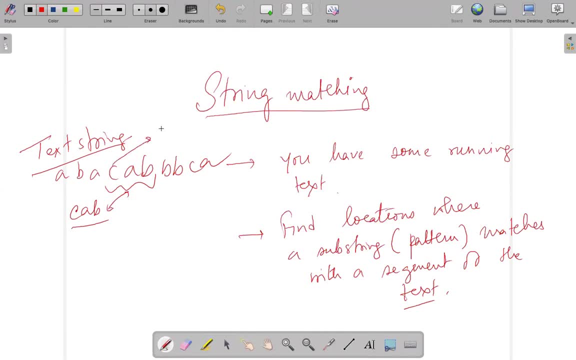 actually returns the point at which the match was found, And also sometimes it returns the boundary Fine. so I guess, immediately, as I have noted this problem, you can think of multiple different areas where this can be used. So, and in fact, this is used in text processing. 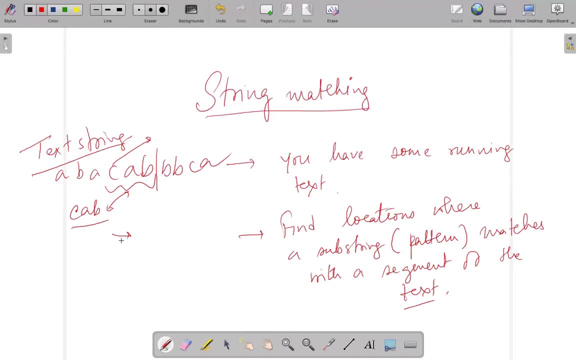 in bioinformatics and many other places. So, for instance, think of a very simple example of finding words in a text document. So string matching- String matching is one of the options by which you can try to find words in a particular text document. 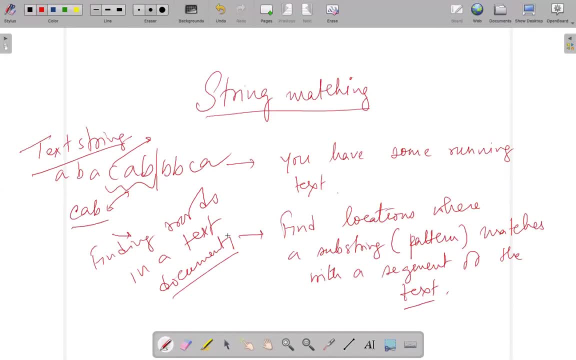 And say: your simple task is, you know, given a text document, you want to find a particular word w and count the number of times it has occurred in the word sorry occurred in the text document. So this is typically also called the frequency of the word. 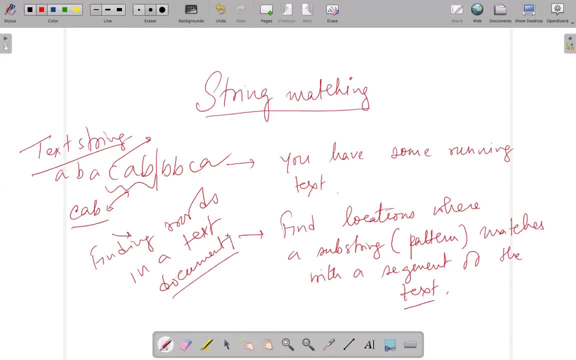 So you find out the word and the frequency In this way. you can find out the word and the frequency In this way. you can find out the word and the frequency. In this way. you might want to find out the word and the frequency of all the words in the text document. okay, 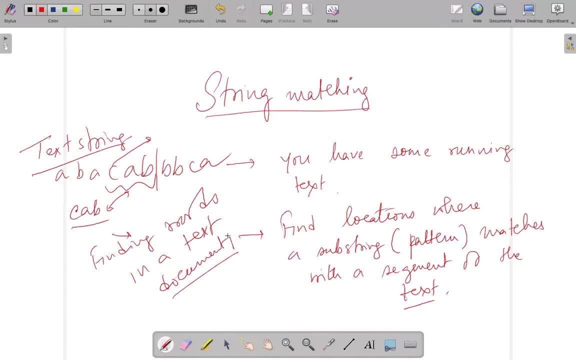 And string matching is one of the ways in which you can achieve this. So I would suggest that, once I have taught you this algorithm, try to do the exercise that I just now mentioned: Find A word And the number of its occurrences in a running text document. 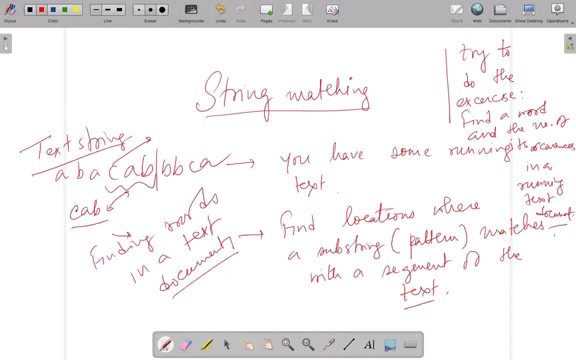 And do it for all words. All right, so you have a word frequency table. okay, so you are given, say, a text document. your task is to find out or compute a word frequency table where each word should appear in the running text and the frequency is the number of times the word has occurred in the text. 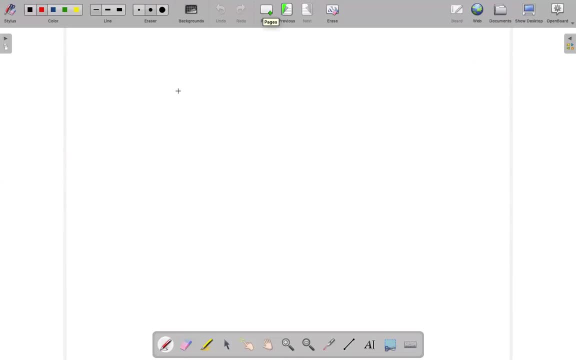 okay, so we will talk about two different algorithms. the first one that we will discuss today is called the Rabin-Karp algorithm, and the second one that we will discuss next day is called the North-Morris-Pratt algorithm, or more popularly known as the KMP algorithm. 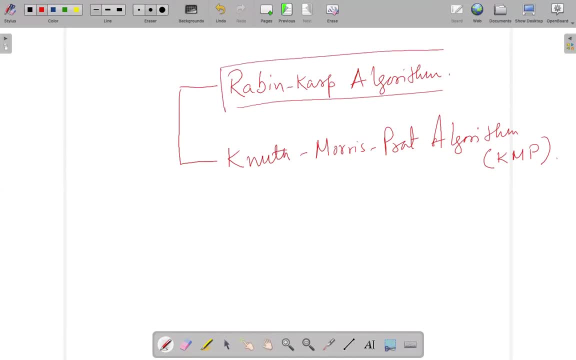 so I have chosen this particular algorithm as the first one, because this continues from your previous topic that I taught you on hash tables. okay, you will see that how hash tables, or hashing in general, can be used to achieve real world problem solving, like string matching, okay. 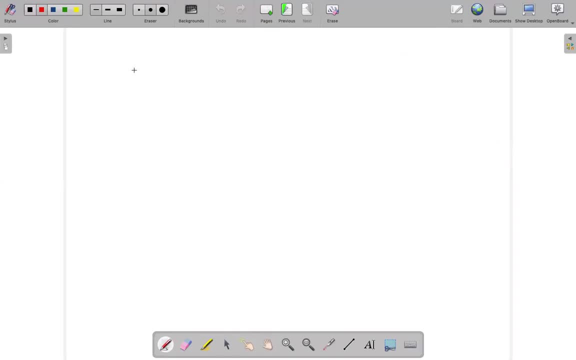 so the idea is as follows: so you are given a text string and you are given a pattern to be found in the text string. okay, So this is the task. these are your two inputs. fine, so what you do is you calculate the hash value. so this is the top level idea: hash value for the pattern right and for each of the. 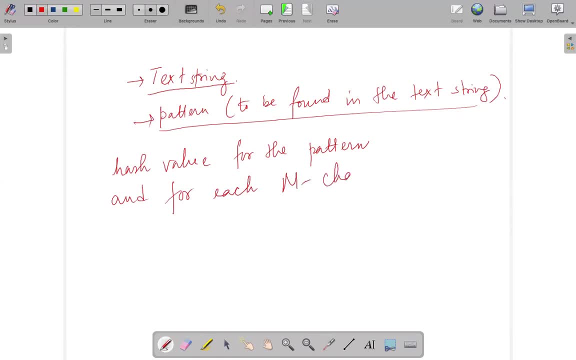 m character sub sequence of the text string. so you have a hash for the pattern and you have a hash for each of the m character sub sequence. okay, So let us talk about hash table. So you have a hash for each of the m character sub sequence. 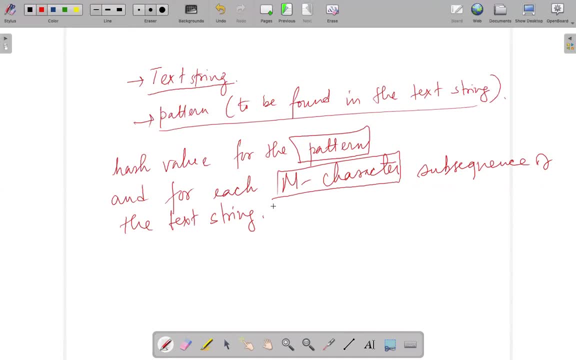 Let us go to the next one sequence of the text string. Now there can be two things that can happen If the hash value are unequal. if the hash values are unequal, the algorithm will calculate the hash value of the next m character. 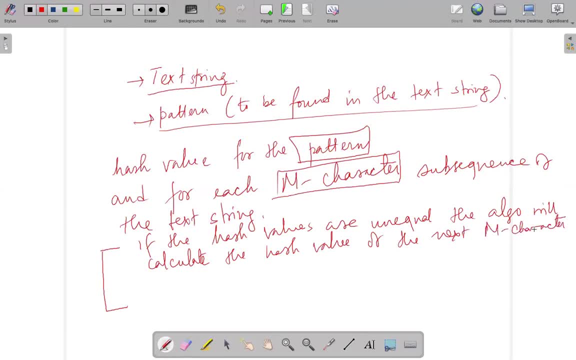 sub-sequence of the text string. If the hash values are equal, then the algorithm will compare the pattern of the text string with the m character sub-sequence, sub-sequence, character by character. So there are two parts in the algorithm. 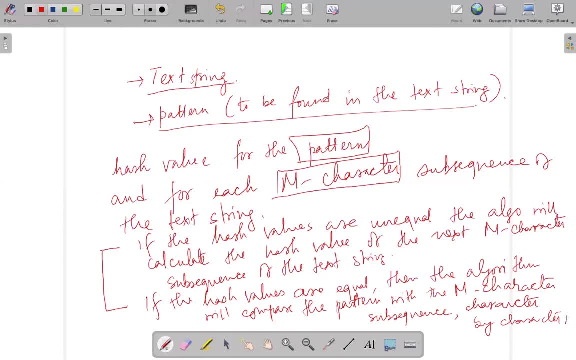 So first part is you compute a hash value for the pattern and you compute a hash value of m- character, sub-sequence of the string, And then if the two hash values are unequal, then you slide. Then you slide One character. 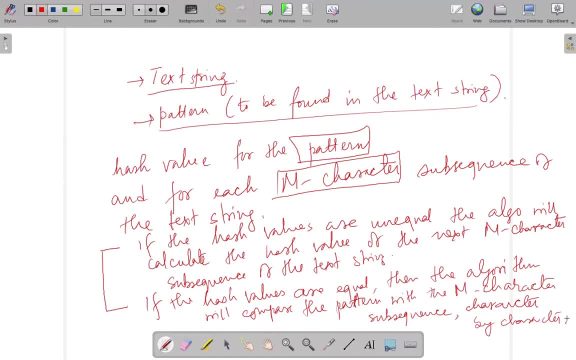 So this is also sometimes called the sliding window. So you slide one character and you take the next m characters compute their hash and compare it again with the hash value of the pattern And you continue this In case if the hash values are equal. 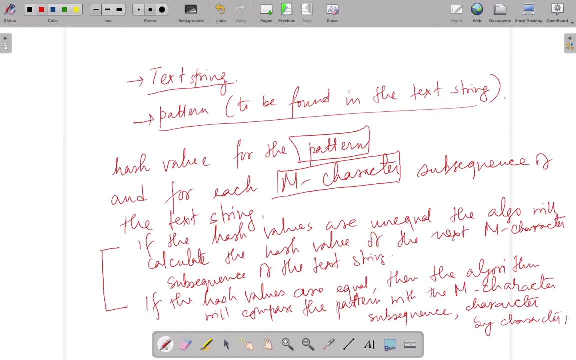 then you know that there is a chance that the m character sub-sequence is going to match with the pattern, And in only such cases you make m character sub-sequence. So this is an explicit character by character comparison. So as you understand, 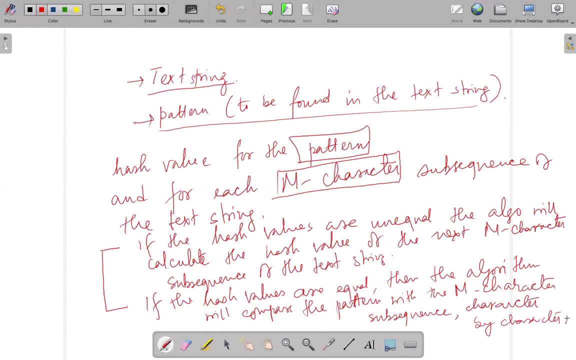 this hashing directly reduces the total number of computations that you need to do. that you would have needed to do if you had to do the whole thing character by character. So the character matching- remember this is required only when the hash values match. 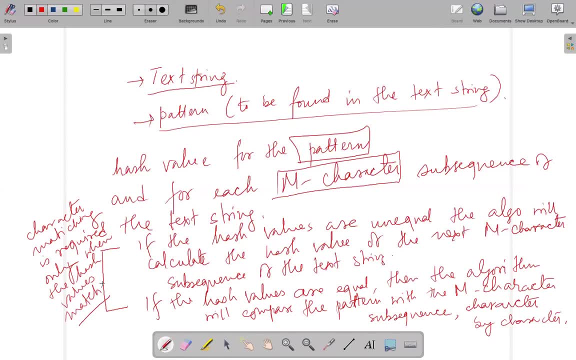 Fine. So this is the only case when the character matching, explicit character matching, is required. Now, if your hash function is very poor, then you will collide a lot and explicit comparisons will be more. However, if your hash function is good, 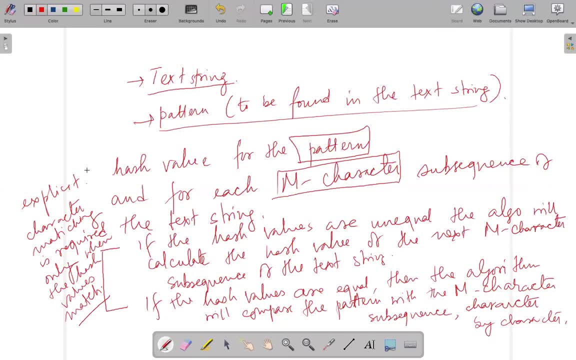 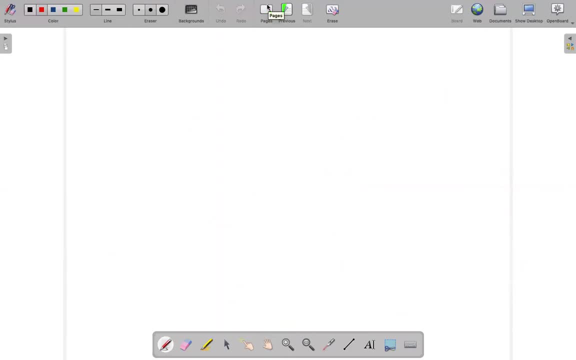 then your collision will be very less and your explicit comparison will also therefore go down. So how do we achieve this? Okay, So let us first try to set up the mathematical aperture. okay for this. So let us consider. 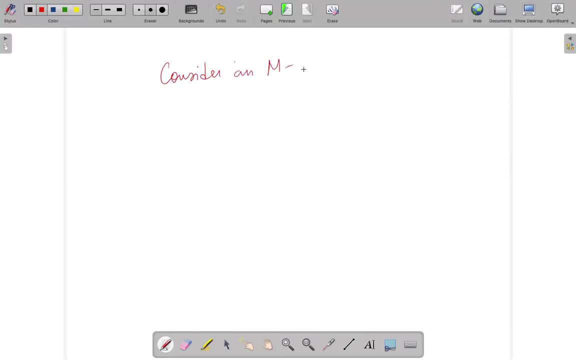 an m-character sequence- okay, as an m-digit. and we Now, as I mentioned earlier, we need to have this one thing that we can use as a f-character sequence. Okay, We can use this as m-digit. So this is e. 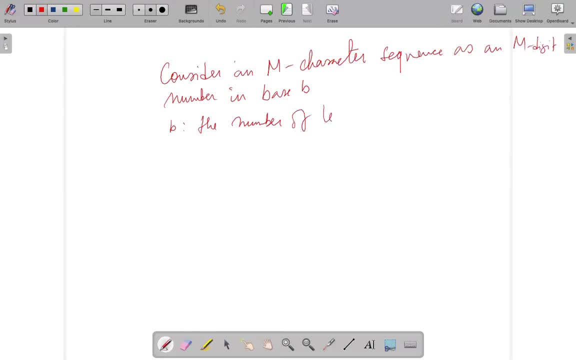 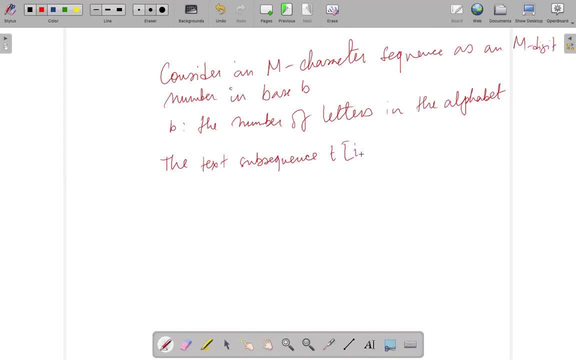 say T I to T I plus M minus 1 is mapped to the number XI, where XI is expressed as TI into B to the power M minus 1 plus T. I plus 1 into B to the power M minus 2, plus, so on T I plus M minus 1, B to the. 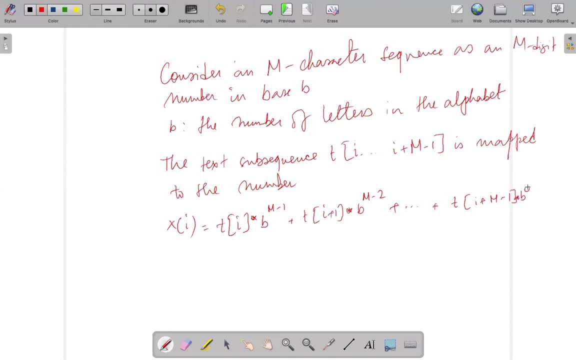 power Z. okay, so now from XI we can compute X, I plus 1. okay, for the next subsequence: you now, in order to do this, we need to find a smart way, right? so every time we cannot do this computation like for every I, we cannot afford to do this. 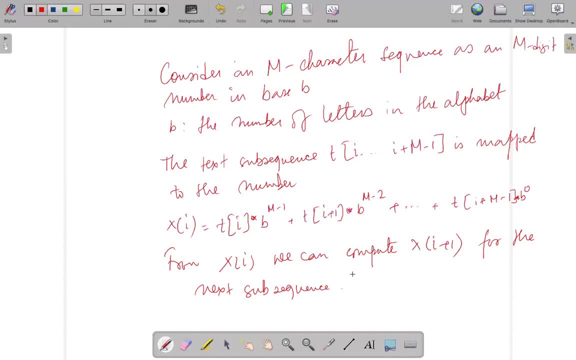 computation. so we will try to have a tricky manipulation of XI in order to obtain XI plus 1 it. So we do the same thing if we take T? I plus M for T? I plus one. so we will try to have a tricky manipulation of XI in order to obtain XI plus one. 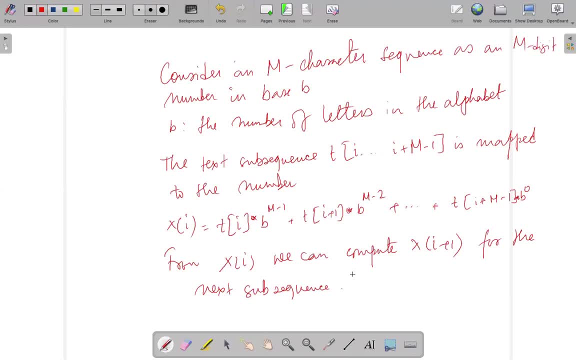 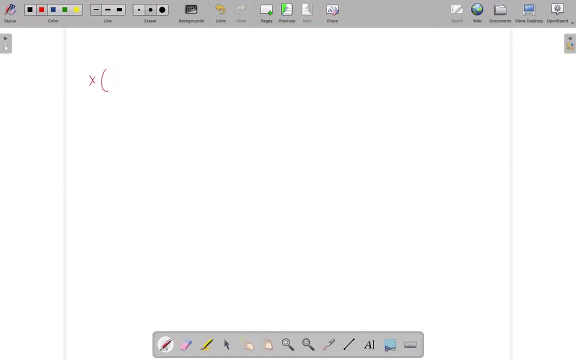 okay and, as I'll show you, this can be done in constant time. so it is very apparent if you see the structure of X I plus 1, so X I plus 1 looks like this: T I plus 1 into B to the power minus 1. sorry, B to the power, M minus 1 plus T I plus 2. 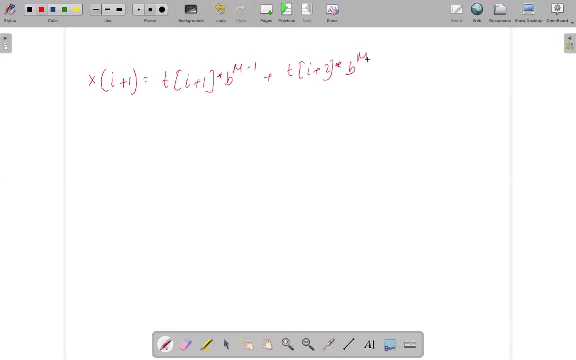 into B to the power M minus 2, plus up until T I plus M into B to the power 0. okay, so now if you look at these two expressions, X I and X I plus 1, it it becomes immediately apparent that X? I plus 1 can be obtained as X I into B. 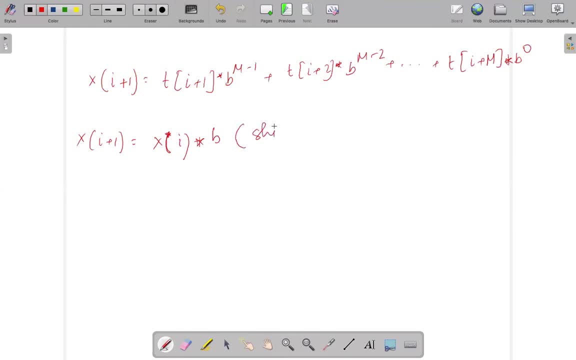 minus 2 into B plus 1. so, Deb, 이게 far pinned down. so I'm going to split, if you are, as if you are shifting left one digit minus TI into B, to be M subtract leftmost. now, if, if you are now ordained to B, to the power 1, if you and I are not in turn, you mind you will have to grey. what is it? as if we are waiting straight away. if you are. 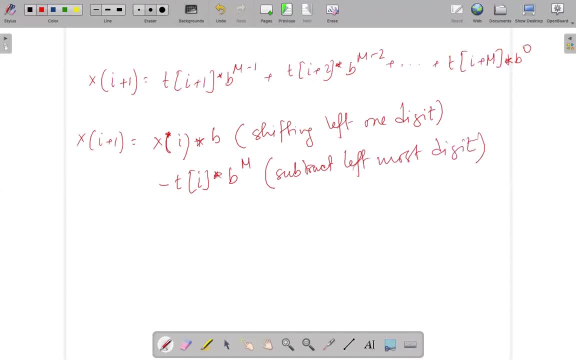 digit. okay, plus T I plus M, add the right most new digit, right. so in this way we can slide over and from the previous X I we can compute the next X I plus 1 in just constant time. okay, now, if M is very large, then these numbers- X I, X, pi plus 1, etc. can be very, very large. 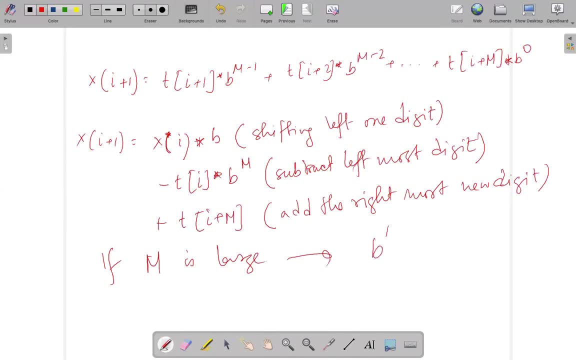 okay, So, in general, Bm is large, could be very large. so therefore, what we do is we always express these numbers as modulo Q. okay, where Q is a prime, fine. So this is actually easily doable because of the following properties of the modulus function: okay, So I guess. 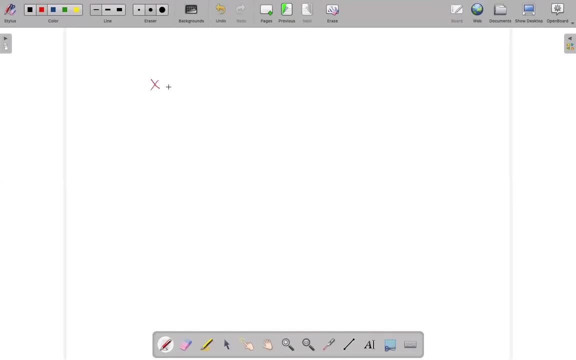 all of you would remember from your last two days that X mod Q plus Y mod Q mod Q is nothing but X plus Y mod Q. okay. Similarly, X mod Q mod Q is nothing but X mod Q. Okay, as simple as that. So for these two reasons, now we can transform. 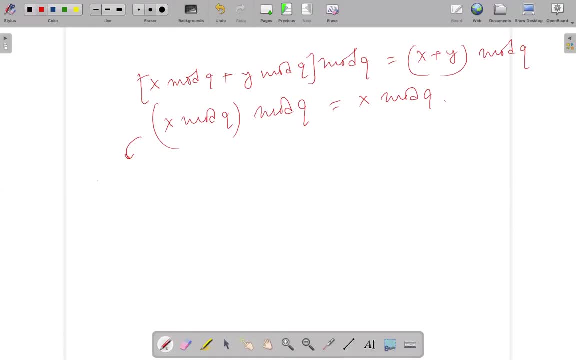 Xi to His which are in the modulo domain: Ti into b to the m minus 1 mod Q plus. Ti plus 1 into b to the m minus 2 mod Q plus so on and so forth. Ti plus m minus 1 mod Q. 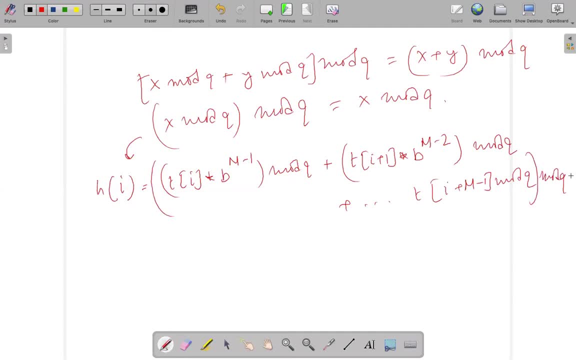 mod Q. Okay, Similarly, Hi plus 1 is Hi into b mod Q minus Ti, into b mod Q minus Ti, into b mod Q mod Q mod Q into b to the. And then we put i plus i plus m into i plus m. 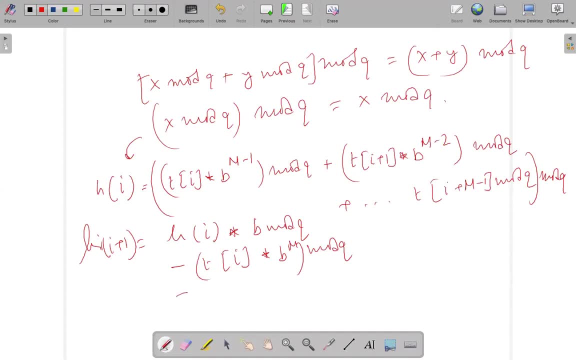 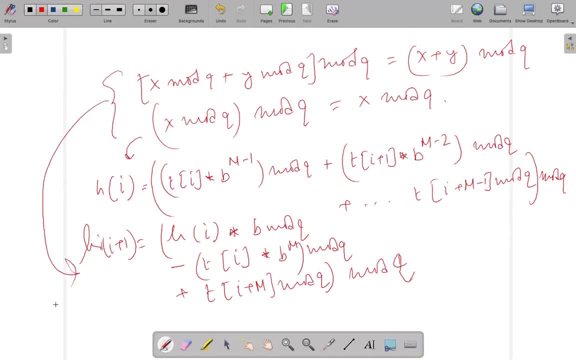 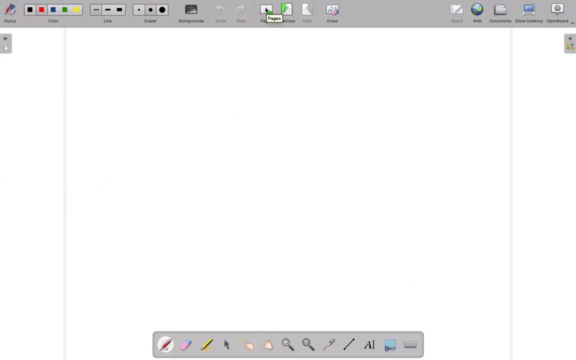 Mod Q, mod Q, mod Q derived. fine, so now, given this, we can write the Rabin curve algorithm. given this transformation, we can write the Rabin curve algorithm. so the algorithm is very simple. once you have written this formulation properly, you let us see that n is equal to the length of the text string. 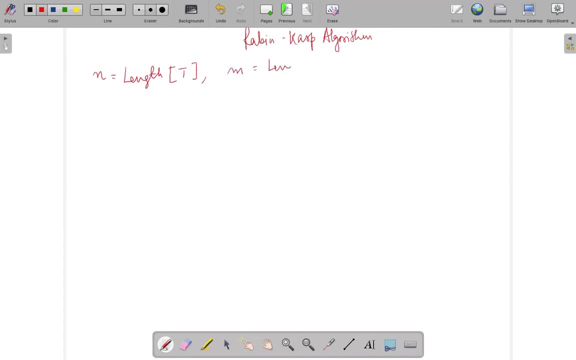 and M is the length of the pattern. let us define the length of the text string, and M is the length of the pattern. let us define H as B, to be M minus 1 mod Q. let us say P is equal to 0 and T 0 is equal to 0. okay, now for. 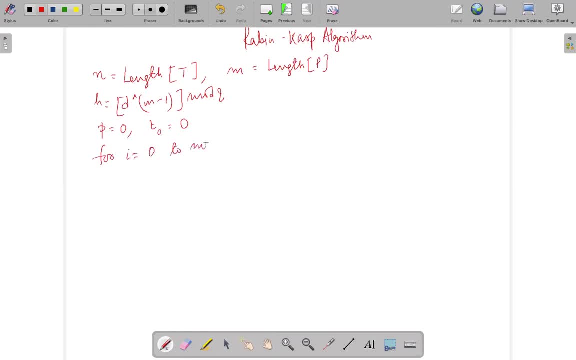 I equals 0 to M. we compute the first two things: P is equal to D into P plus the I mod Q, and T 0 is equal to D into T 0, zero plus T I mod Q. so this is the hash of the pattern and this is the hash of the first. 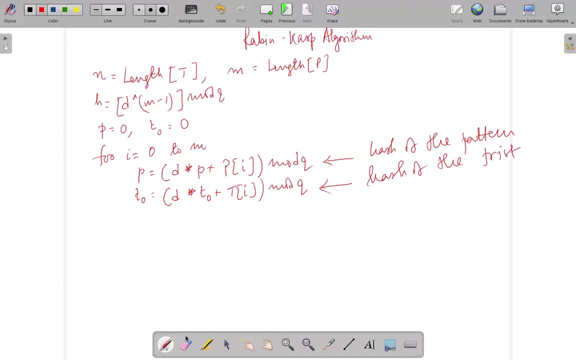 sorry, the first in characters of the string T right now for s equals 0 to in minus M. since we have already consumed the first M, so we run from 0 to N minus M. if P is equal to T. if this is true, then if P 1. 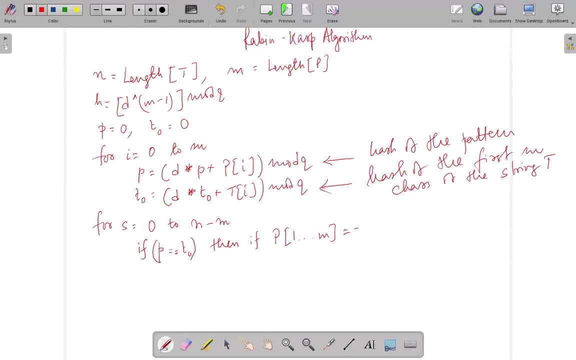 to M is equal to T, s plus 1. through s plus M, we trigger pattern found in the first string and at shift: yes, okay, so these part actually you can interpret as an explicit character by character matching: you, you, you, you, Fine. If this is not true and if S is still less than N minus M, then what do we do? We? 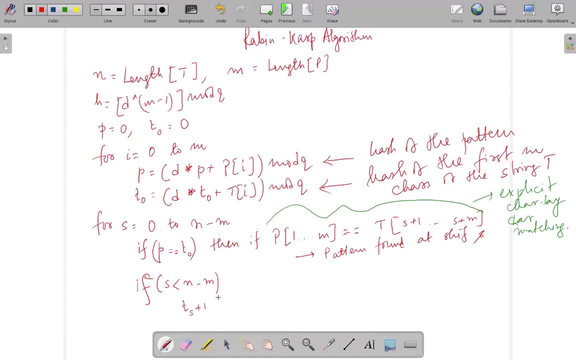 set T S plus 1 as D T S minus T S plus 1 into H plus T S plus M plus 1.. Okay, So this is how you try to now. So this T S plus 1 will in constant time compute the. 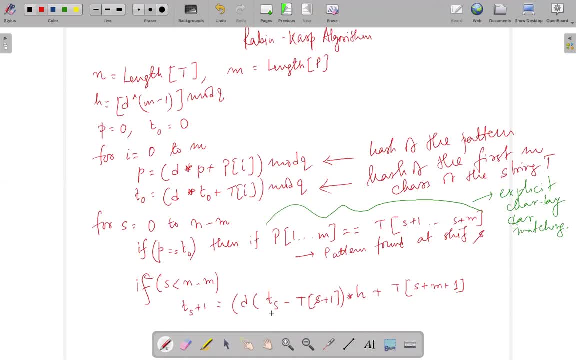 next hash from: given the value of T S right. So the algorithm is as simple as this. Now let us take a small example and check out. Okay, So this is how you try to now. So this is how you try to now. So this is how you. 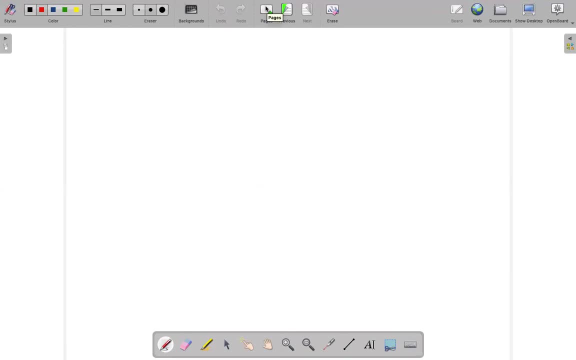 find out how it functions. Let's say we have a string like this: You. let us say we have a string of this form, okay, and let us say our Q is 13 in this case, okay, and we want to calculate the you, the hash for. 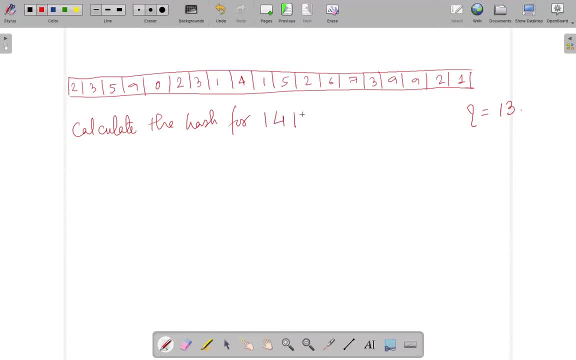 the pattern: 1, 4, 1, 5, 2. right, so that is this one: 1, 4, 1, 5, 2. we want to calculate the hash for this and, as you see, the numbers are between 0 to 9, and so the alphabet here is 0 to 9 and therefore base is 10. okay, which is the number of elements. 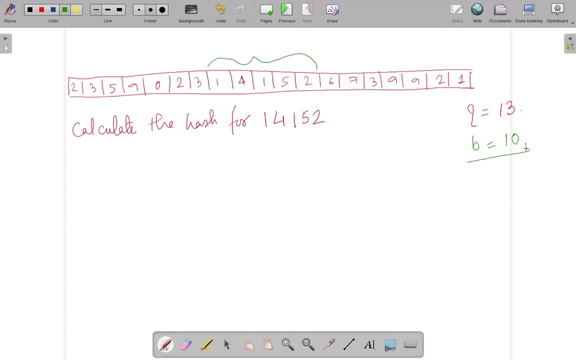 in the alphabet. so, given this, we can compute the hash for 1, 4, 1, 5, 2. if I tell you that the hash of 3, 4, 2, I 3, 1, 3, 1, 4, 1, 5. 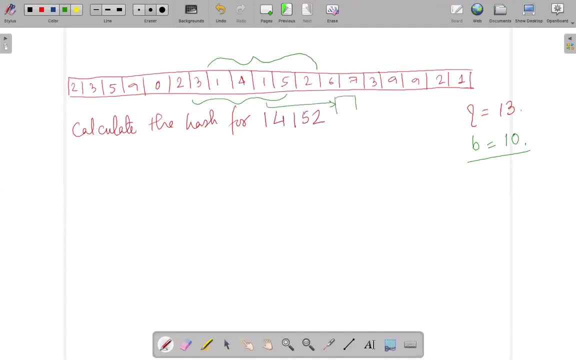 is given to be 7, it would be very easy for you to compute the hash of 1, 4, 1, 5, 2. okay, so let us see explicitly so: hash of 1, 4, 1, 5, 2, 1, 2. 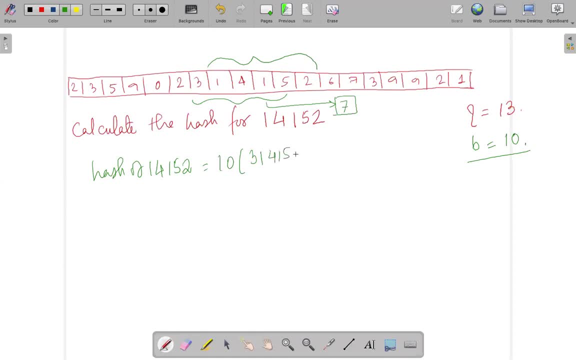 equal to 10 x 3, 1, 4, 1, 5 minus 3x 4 modulo 13 plus two modulo 13, that is eight. okay, so as simple as that. now you see that, as I said earlier, also there could be collisions, okay, and you will see, like, if you keep on computing like this, then 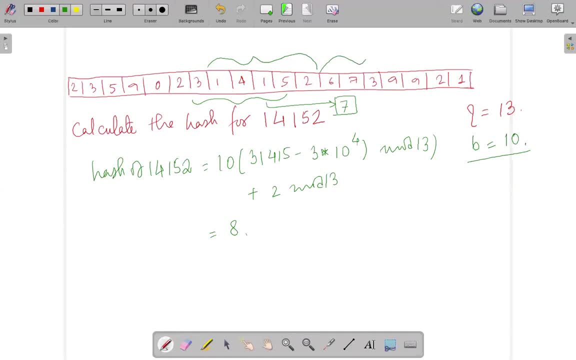 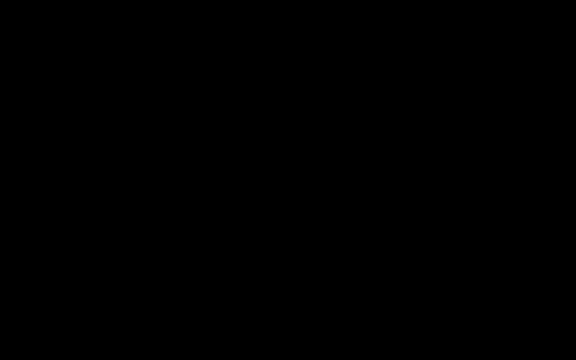 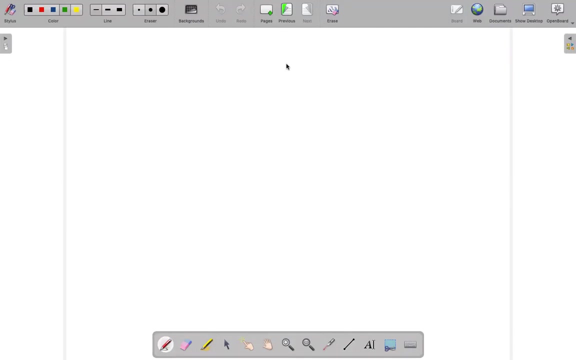 this series- six, seven, three, nine, nine- will again lead you to a hash value of seven. okay, so this is something that you need to be careful. so the complexity of this algorithm is straightforward to calculate. so now you you can see that this is a very complex algorithm and you need to be careful. 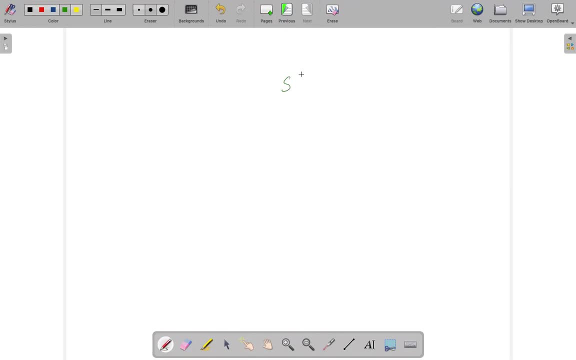 so the complexity of this algorithm is straightforward to calculate. so now you have seen that the variable s that runs right, n minus m times. okay, right, so it goes from- goes in minus m times, the first time being directly compared, and after that it runs in minus m times. now in this: 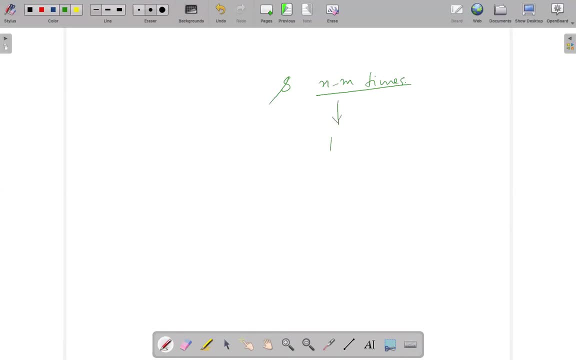 loop like what could be the worst case. the worst case is where kalisha knockers are in every step, every slide. so as you slide the window, in every slide there is a collision. this is the worst case and for each collision, when you have collision occurs, a collision is. 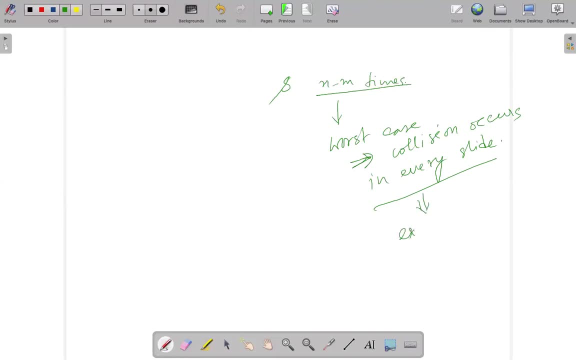 each such collision you will have to do a exact character by character match, right? so there are M characters, so you will have to match M characters of the text string with the M characters of the pattern. so this character by character match will take time. order M: okay, and since in the worst case there can be n.